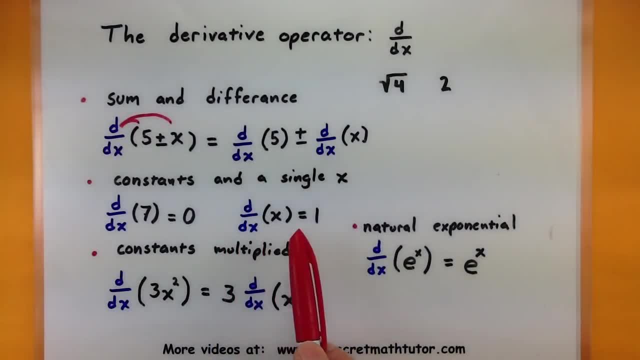 do the, for two in three is x plus x. Oh dibuj elegal interior. How about we plot this: Y times 0 and take the derivative of being a cross: equally zero. That's just zero, so just zero. Now, keep that in mind, that it's completely different if you take the derivative of a single x. That 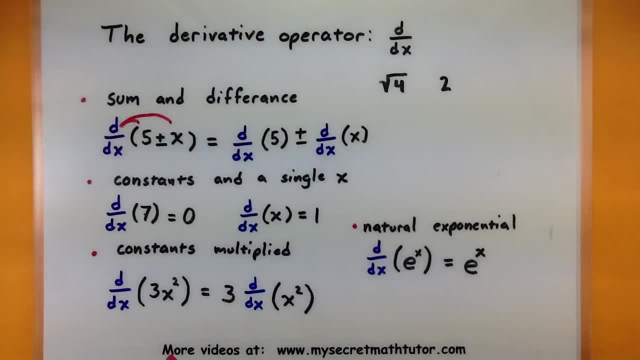 derivative is actually one. When we get to the power rule, you'll see what we do for higher powers of x, like x squared and x cubed. But know that a single power, you get one. all right. Now we also have a rule for what to do when constants are multiplied by something. So think of 3 multiplied. 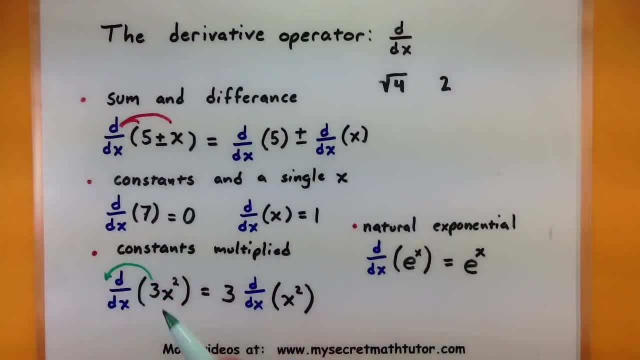 like this, we can actually move that constant out in front of our derivative. So then I'm looking at three multiplied by the derivative of everything else. Now this looks like it's almost a similar rule to this one up here. After all, they both deal with constants, but they are different. 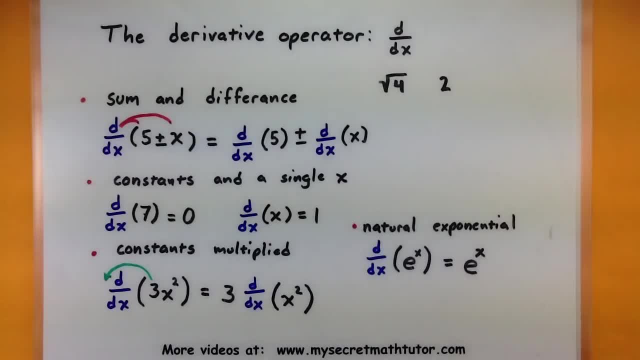 Remember, in this one we have a constant all by itself, so it's a single constant, and this one it's a constant multiplied by something, so it moves out front. okay, All right. and the last of our basics is a really, really neat one. This is when you take: 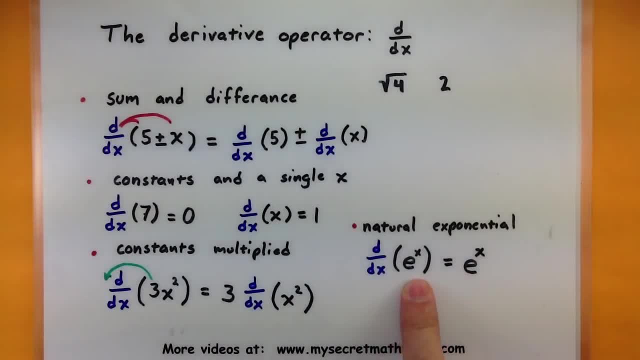 the derivative of a natural exponential, so e to the x. When you take its derivative you get the same thing back, so it doesn't change it. So this is a really handy one, and it's why you often like to see e to the x in a lot of your calculus problems. 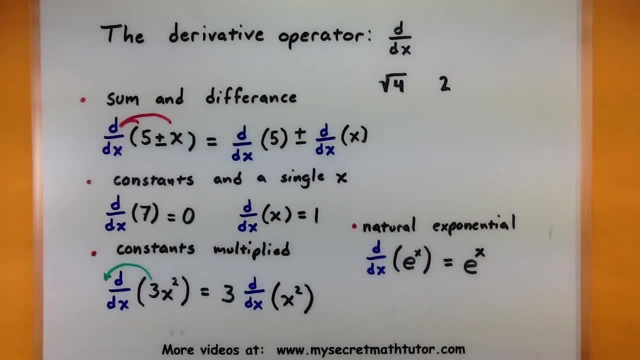 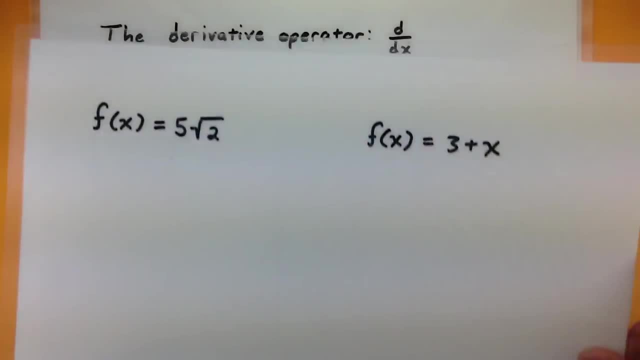 because you know its derivative is just the same as itself. All right, so let's play around with these basics by looking at lots of different examples and see how it works. okay, All right, let's do this first one I have. the function f of x equals 5 times the square root. 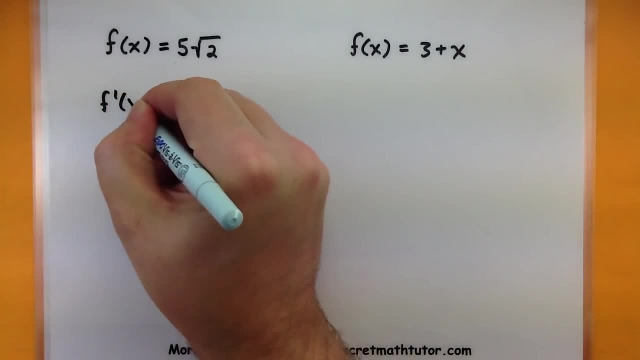 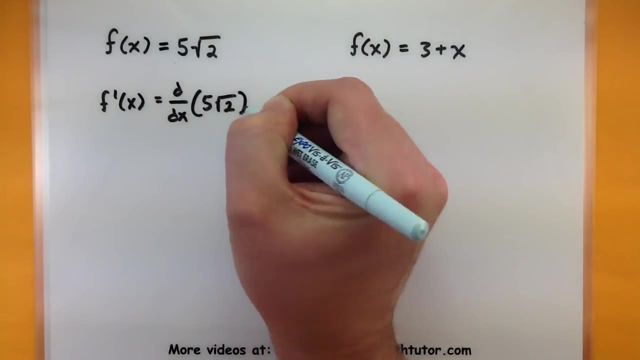 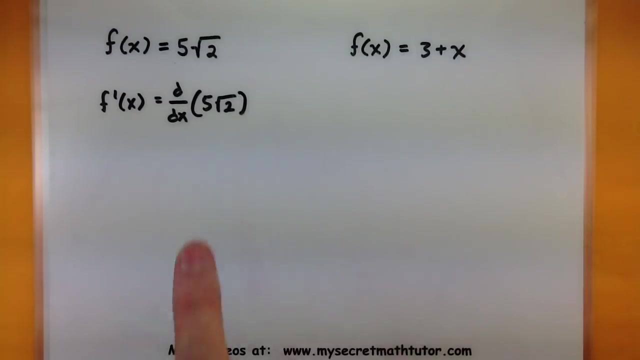 of x. I'm curious: well, what is the derivative of this function? So I want to think what happens when I take the derivative of 5 times the square root of 2, okay, Now think very carefully about what's going on here. This, since there is no x in it whatsoever, is simply a constant. 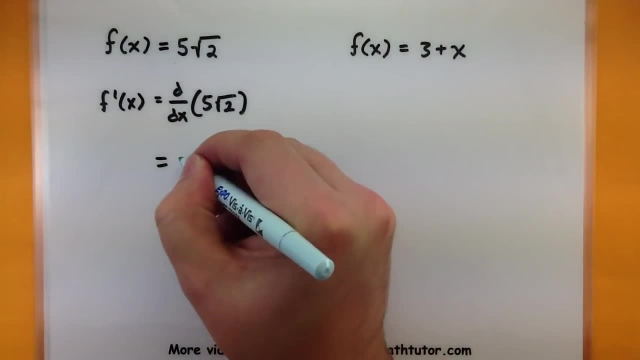 and, of course, according to our basic rules, the derivative of a constant is 0. So I can say that the derivative of this function, f, is 0, just like that. All right, let's do something with a few more things in it. 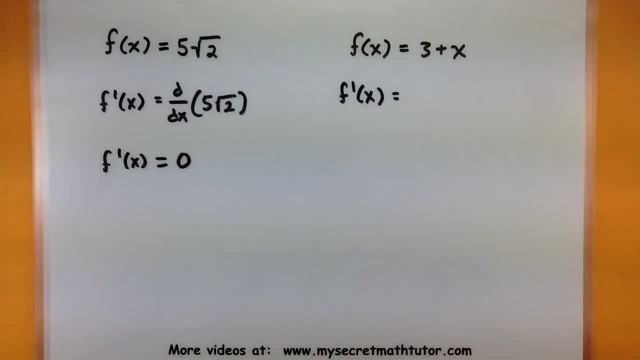 In this next one, we want to take the derivative of 3 plus x. So we want to take the derivative 3 plus x. okay, Now notice how this one has two different pieces to it, and so we want to think of taking the derivative of each of them. 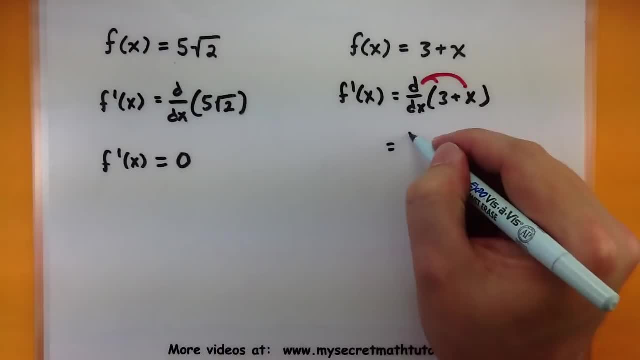 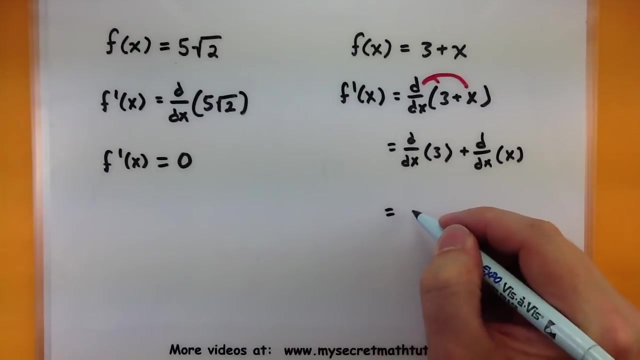 But because they're connected using addition. So now I want to know what is the derivative of 3, and what is the derivative of x. Well, again there's two more derivatives that come right off of our basic rule sheet. The derivative of a constant would simply be 0, and the derivative 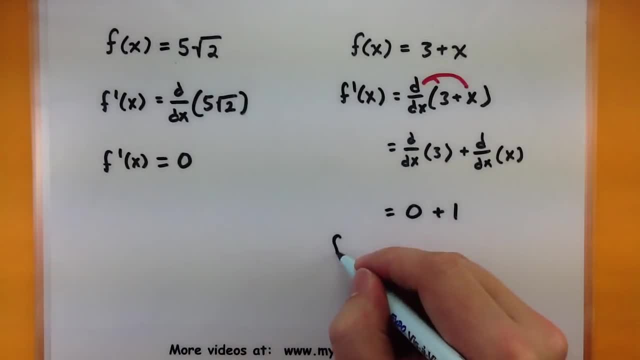 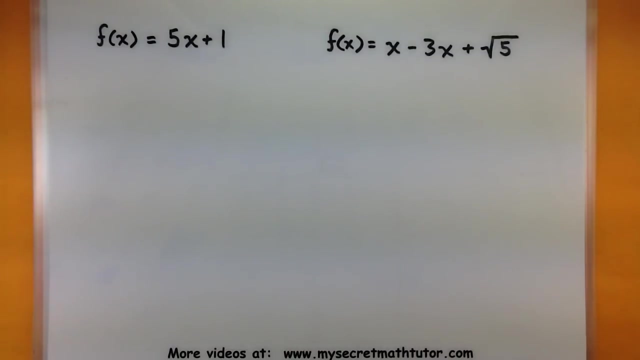 of a single x would be 1.. So I could simplify all of this and say: what is the derivative of f? Well, it's simply 1.. All right, not too bad. Let's look at a few more. Let's see if we can take the derivative of 5x plus 1.. 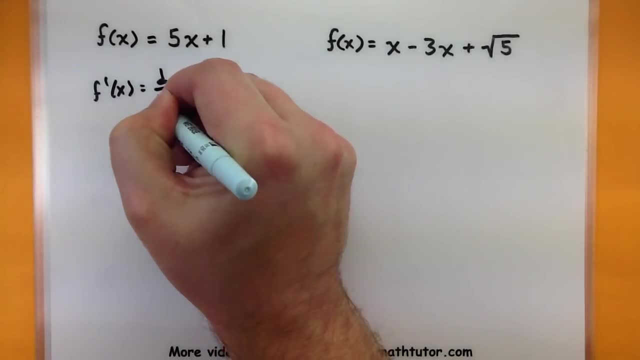 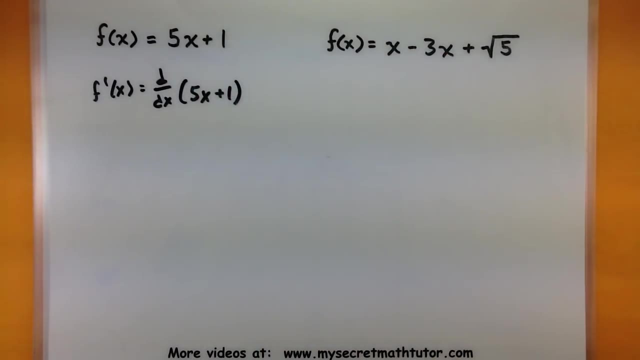 So the derivative of f, we want the derivative 5x plus 1.. Okay, just like before, I can see that I have two pieces that are being combined using addition. So we'll imagine taking our derivative operator and putting it on each of those pieces. 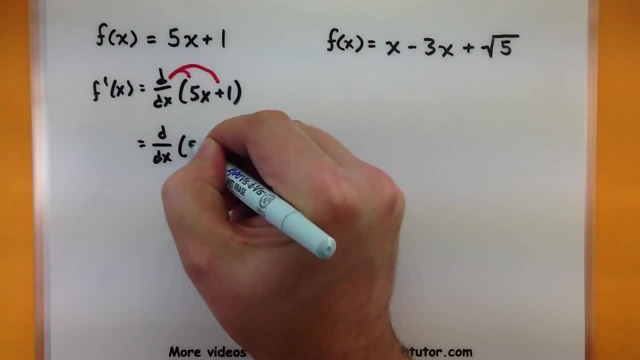 So now we want to know well what is the derivative of 5x and what is the derivative of 1? Now, in this first little piece I have a constant multiplied by x. So I'm actually going to take this 5 and move it out in front of my derivative operator. 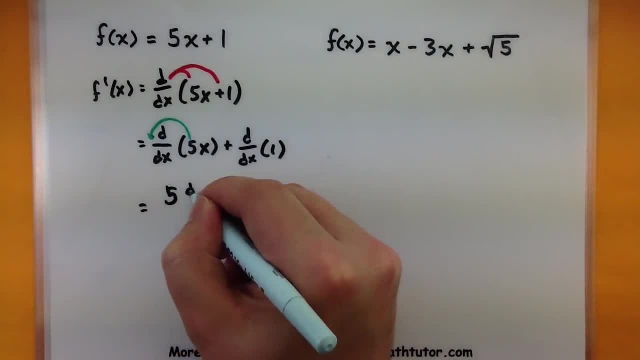 So 5 times the derivative of x plus the derivative of 1.. Okay, and now I have my derivative on these nice little single components here and we can take the derivative of each of those. So 5 times the derivative of x is 1, plus the derivative of a constant 0. 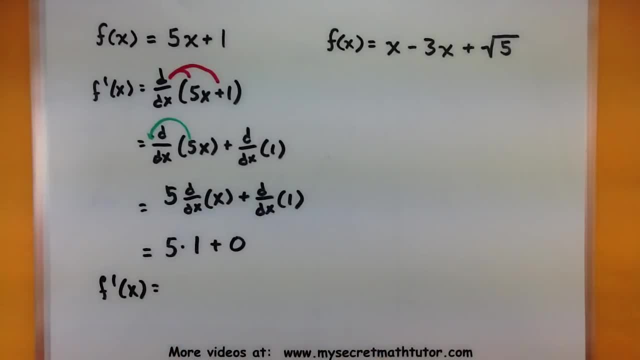 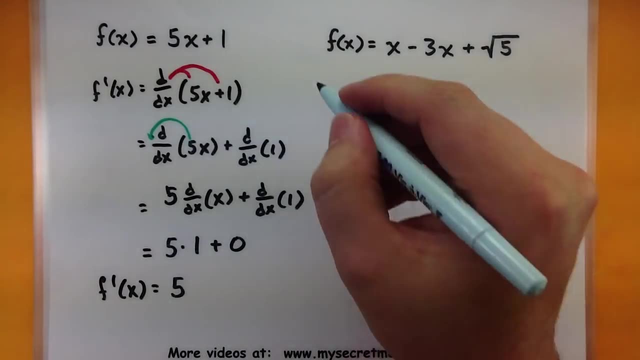 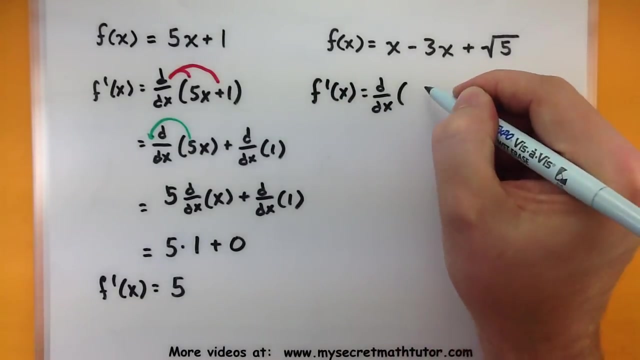 So I know that the derivative for all of f is simply 5.. All right, not bad. This next one has a bunch of different pieces to it. Definitely put your thinking caps on and see how we go through this one. So we need the derivative of x minus 3x plus the square root of 5.. 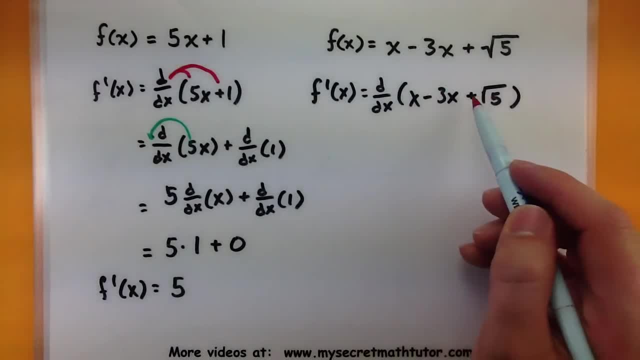 Okay. so even though I got three pieces, they're all connected using subtraction or addition. Let's take our operator here and put it on all of those pieces. So now I'm looking for the derivative of x minus the derivative of 3x and the derivative of the square root of 5.. 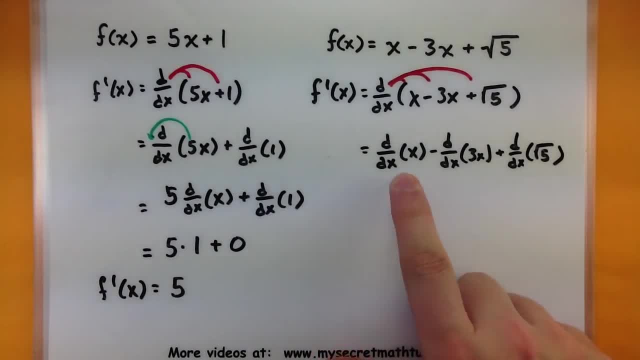 Okay now, two of these aren't so bad. The derivative of x is 1 and the derivative of a single constant is 0. This one, we have a constant multiplied by an x, So we're going to move that constant out in front of its operator. 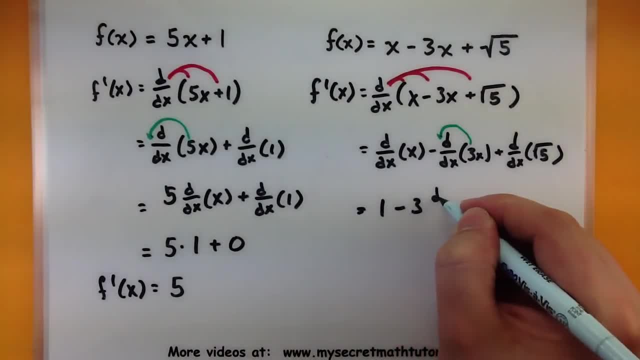 So derivative of x is 1 minus 3.. So we still need to take the derivative of x plus 0.. Okay, so now this is the last derivative I have to do And of course, the derivative of x is 1.. 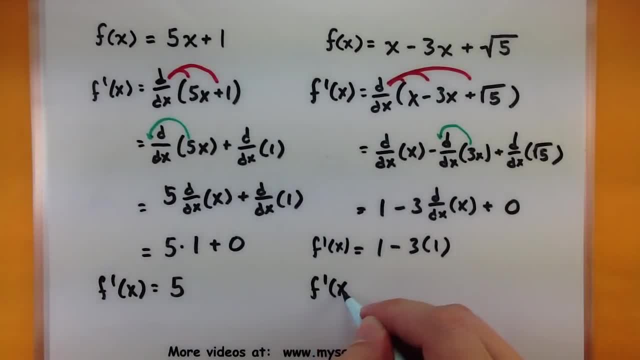 All right. so what do we really have left? So the derivative of f is 1 minus 3 or a negative 2.. All right, looking good. Hopefully it's starting to get a little bit more solid. Let's look at one last example and we'll see how it goes. 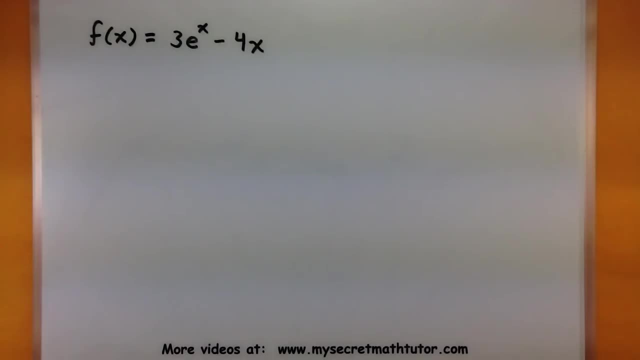 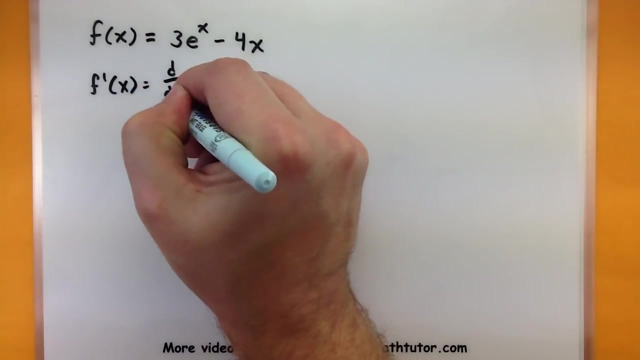 This last one I have. f of x equals 3 times e to the x minus a 4x. All right, so our derivative of f. We need to figure out the derivative of 3e to the x minus 4x. 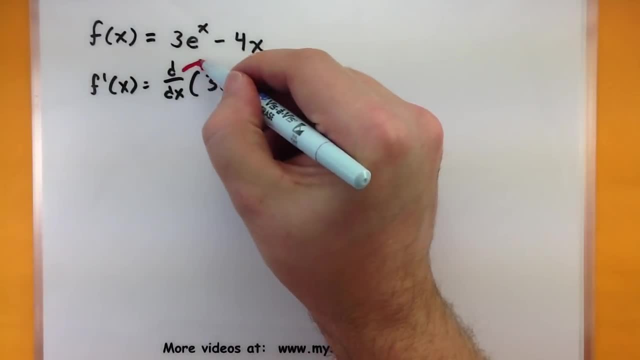 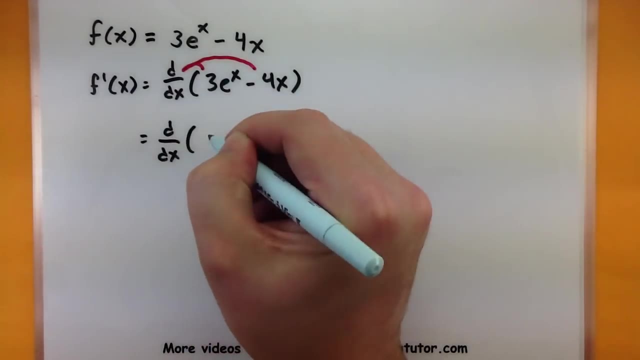 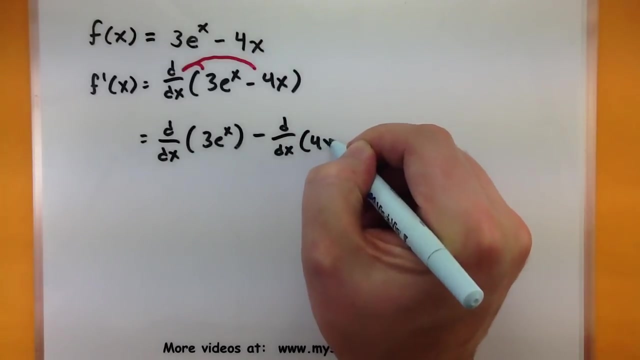 All right, so we'll start off by taking our derivative operator, putting it on each of the pieces. So now we're looking at the derivative of the first piece minus the derivative of the second piece. Okay, each of these have a constant multiplied by something. 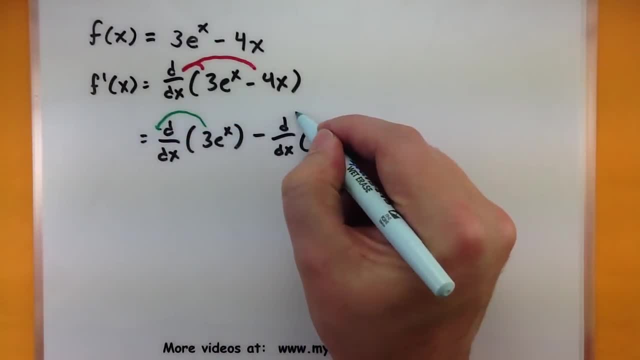 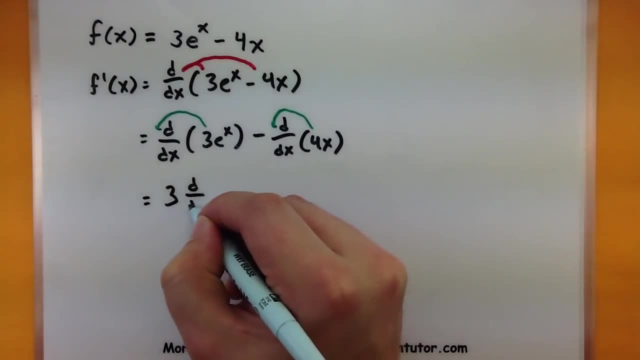 Constant multiplied by something. So we'll move each of these constants out in front. So 3 derivative of e to the x minus 4x, 4, the derivative of x. All right now we can take care of each of these.